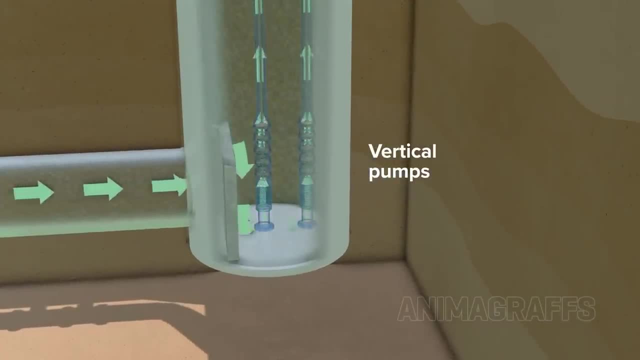 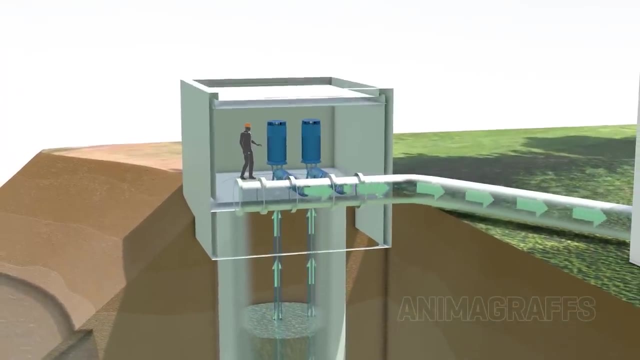 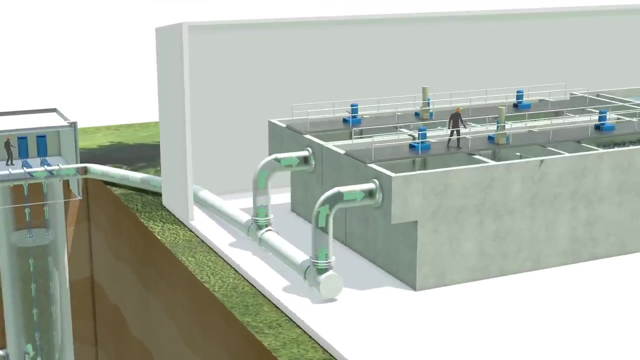 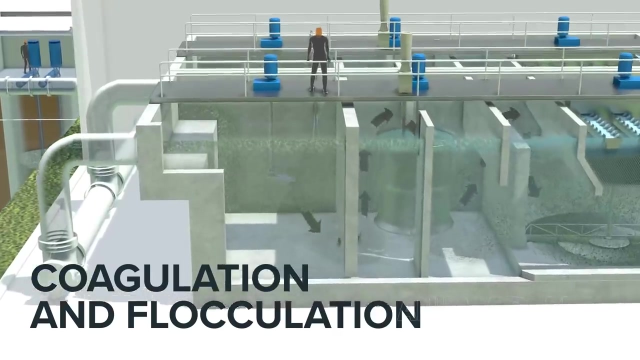 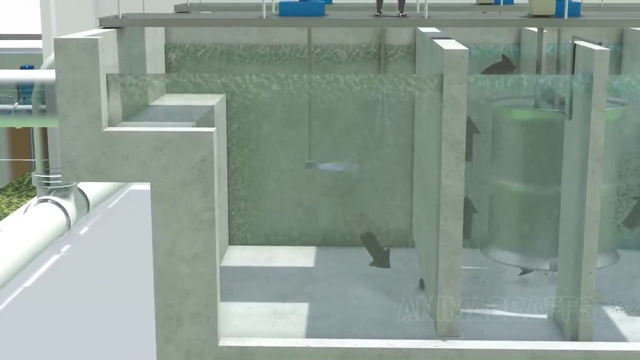 A lift house with vertical pumps draws water from a well and into the treatment plant. The purification process starts with coagulation and flocculation. Particles suspended in water, like clay, sand, and some larger organic particles such as algae, have an inherent electric charge. 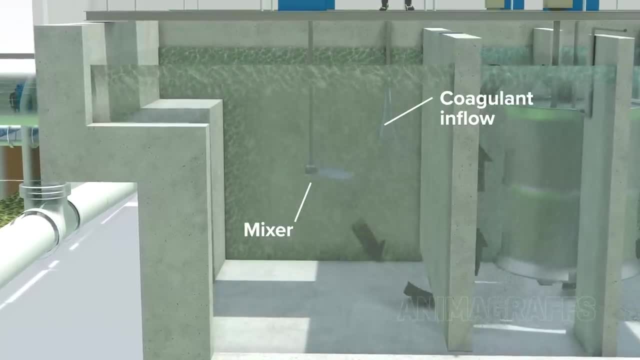 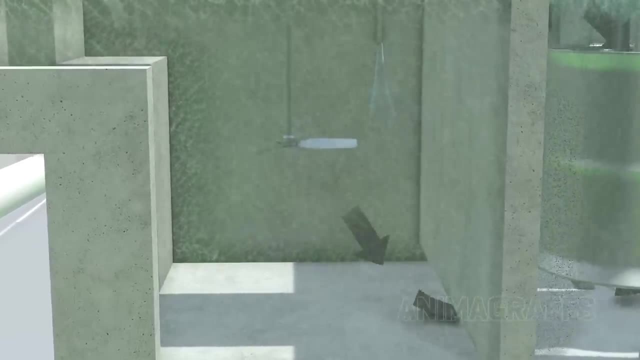 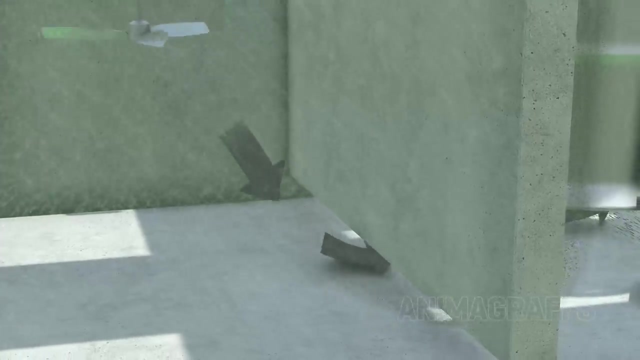 that causes them to repel each other. Coagulants are substances with opposite electric charge that neutralize these particles and encourage them to stick together into clumps called flocc. The coagulant and water is vigorously mixed and flocc clumps start to form. 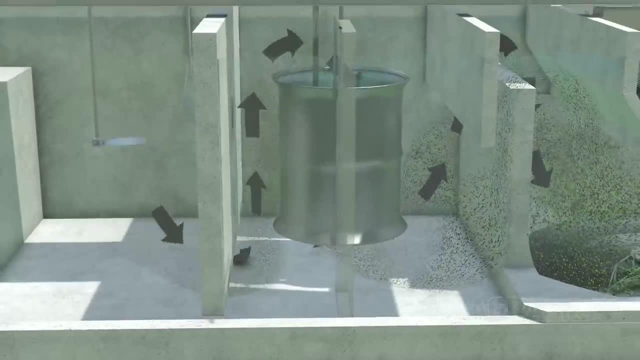 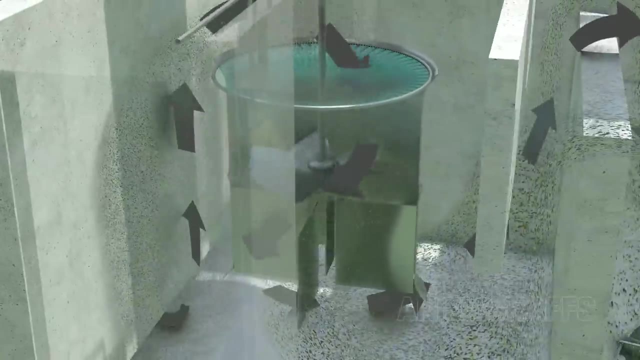 To make flocc particles heavier and therefore even easier to eventually settle out. micro-sand is used to create a coagulant. Micro-sand is added as the water is drawn through a special mixing tube with a polymer to help the sand stick. 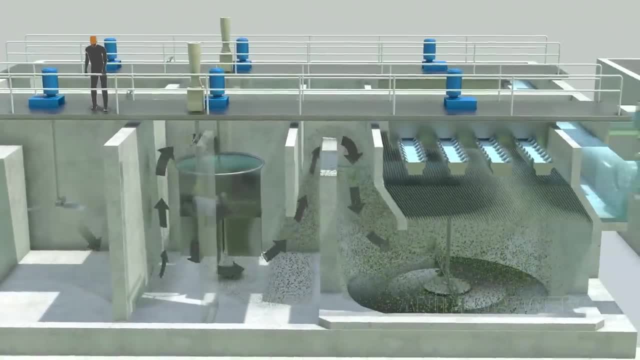 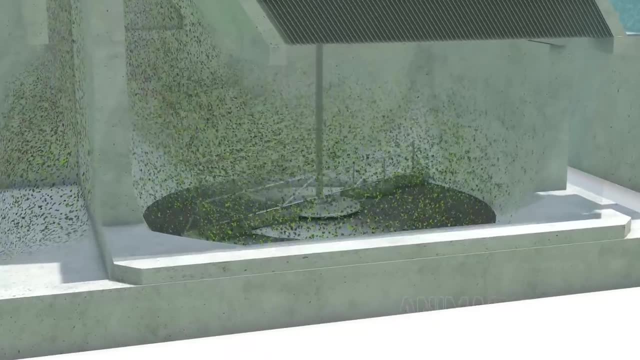 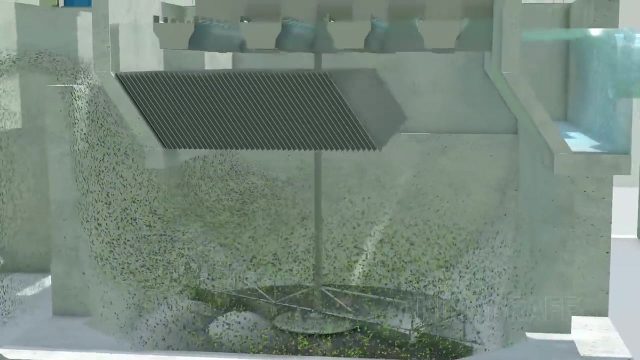 The now flocculated water flows through a set of baffles to slow its turbulence for the settling process. As the water travels upwards, heavy flocc particles quickly settle to the bottom of the tank. Any remaining suspended particles collide with an array of angled plates and slide down to the settling zone. 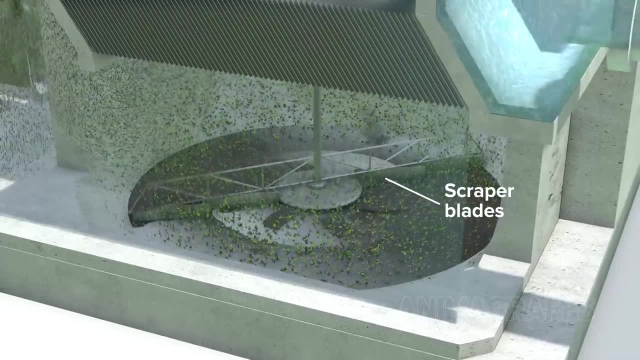 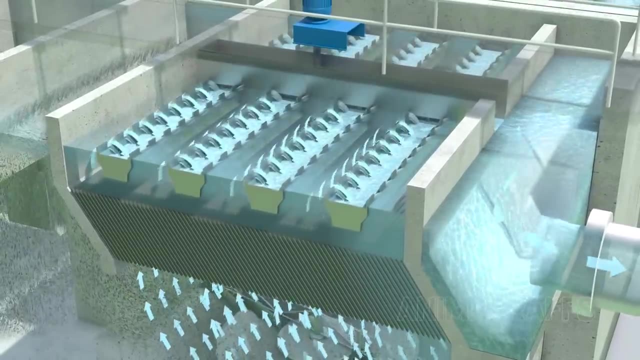 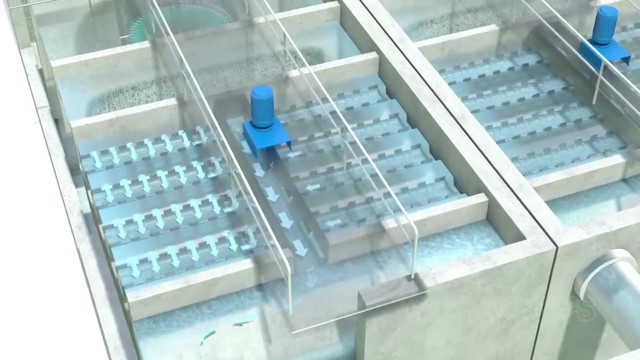 Slowly rotating scraper blades continuously remove the combined sludge and sand layer from the bottom of the tank, while clarified water flows upwards into collection troughs. At this stage, the water already looks clear and a lot less cloudy. Now it's on to ozonation and filtration. 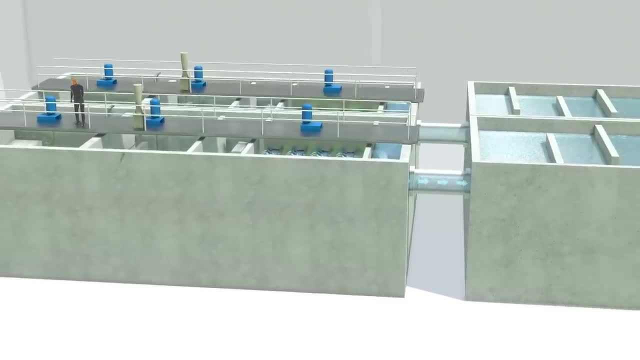 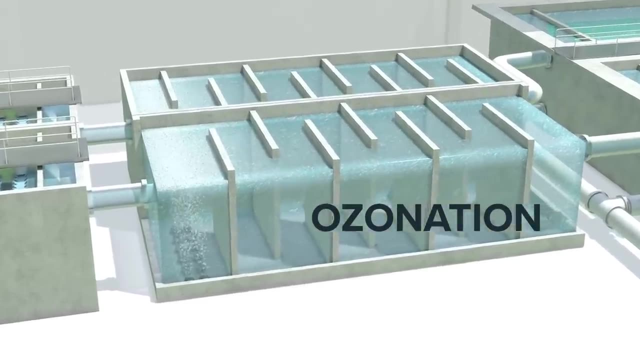 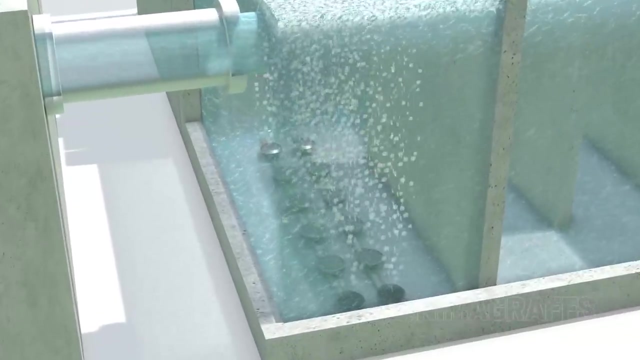 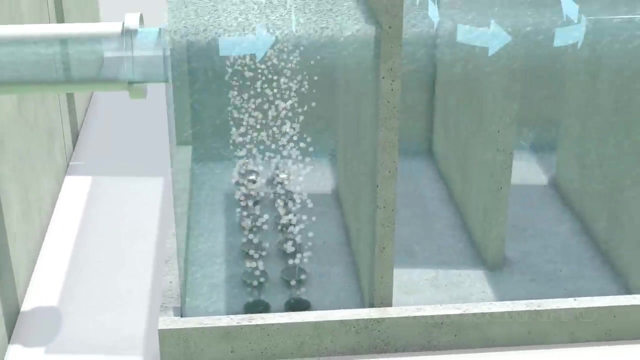 The water is then filtered to treat microscopic taste and odor causing agents. These can include inorganic elements such as iron or sulfur or harmful bacteria and viruses In the ozone tank. ozone gas bubbles are injected into the flowing water through diffusers. The tank is divided, which slows the flow and gives the water a longer path with more time. 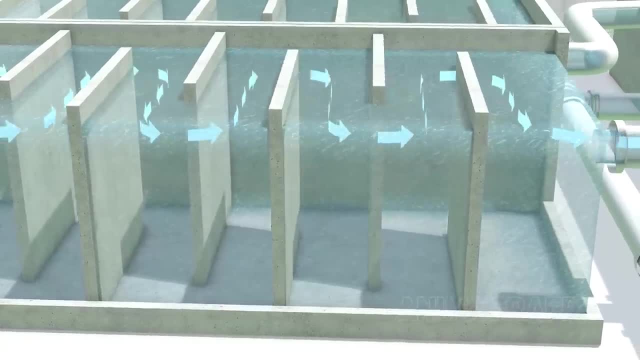 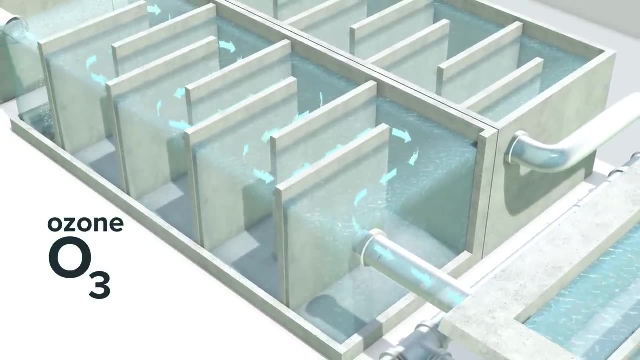 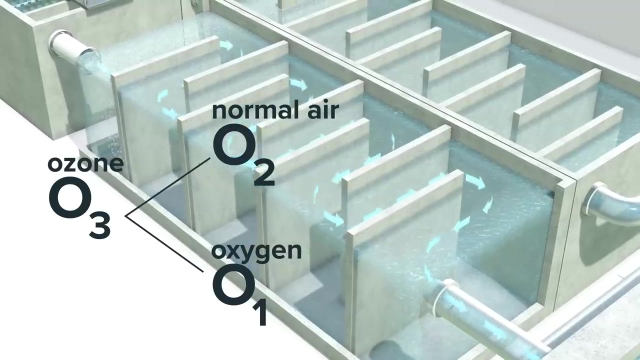 to do its job. An ozone gas molecule is made up of three oxygen atoms. The normal oxygen we breathe has just two oxygen atoms. When ozone is injected into the stream, the extra oxygen molecule can bond with contaminants or oxidize them, with various desirable results. 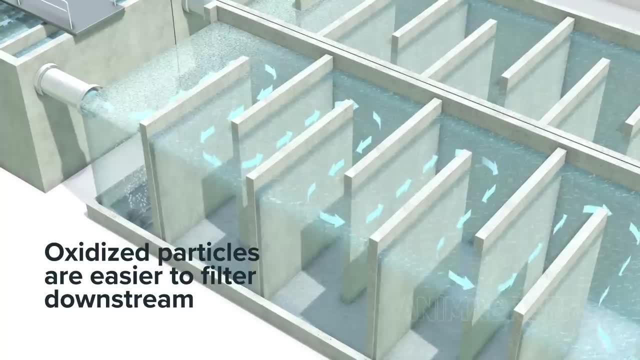 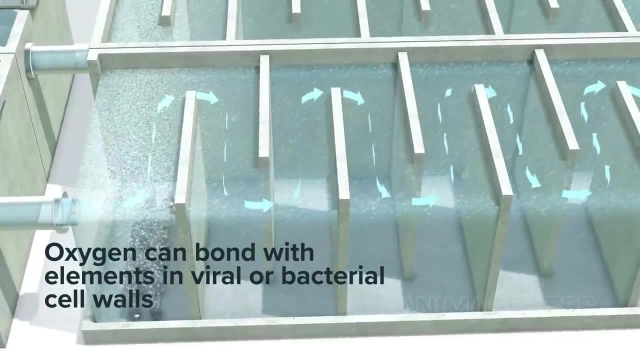 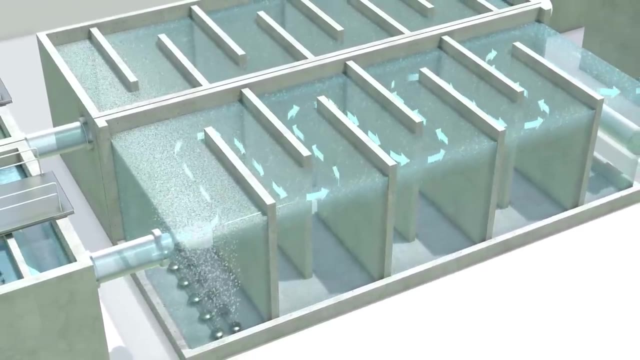 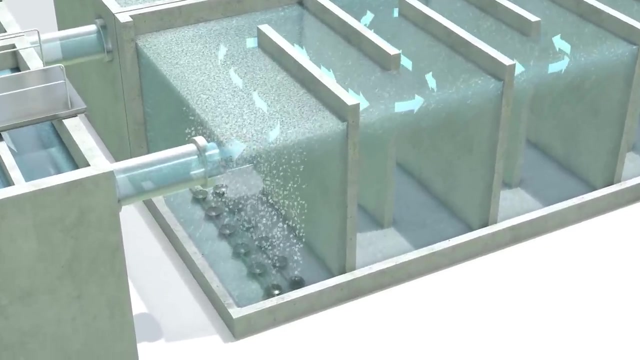 For example, oxidized metals have a weaker bond with water and are therefore easier to extract. Oxygen also bonds with elements in virus or bacteria cell walls, disrupting their function and altering their surface charge for easier filtration downstream. When ozone gives up its extra oxygen molecule, it just becomes normal oxygen. 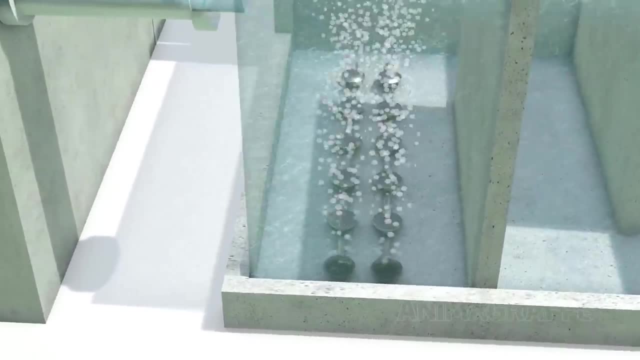 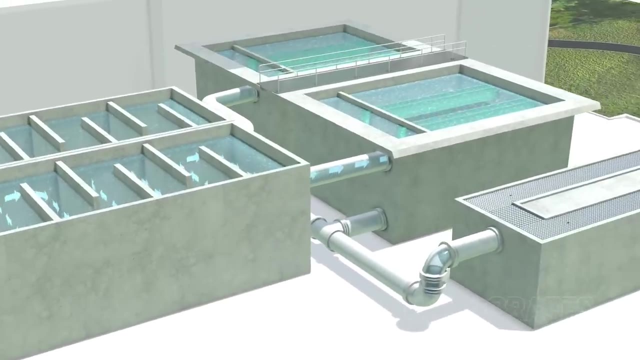 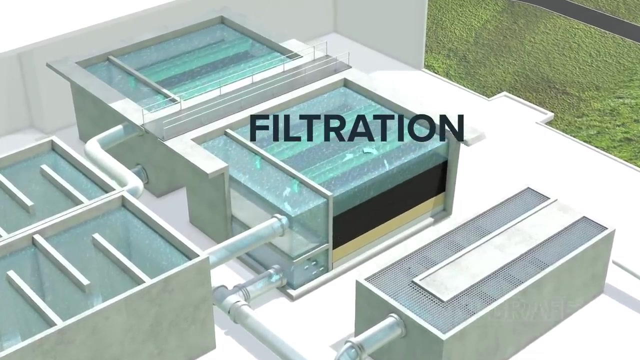 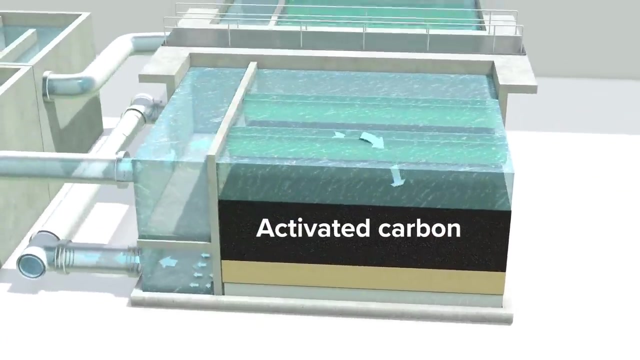 leaving no byproducts in the treated water. unlike other purification methods, such as chlorination, The water flows to the filtration stage to remove the oxidized particles and any other remaining contaminants. Water travels through a dense layered bed of activated carbon granules and micro-sand. 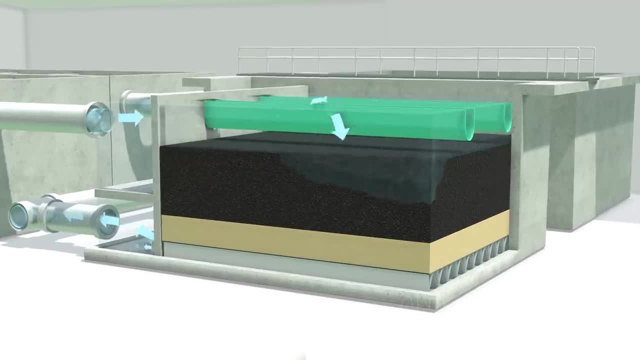 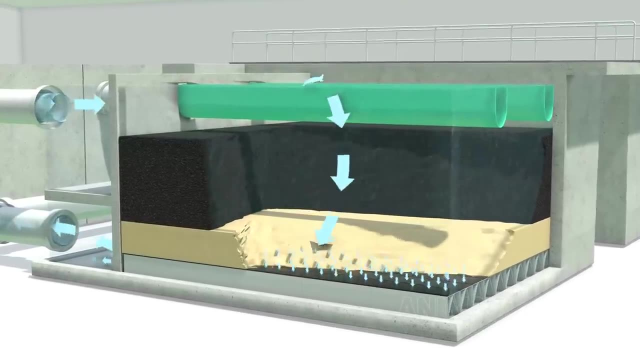 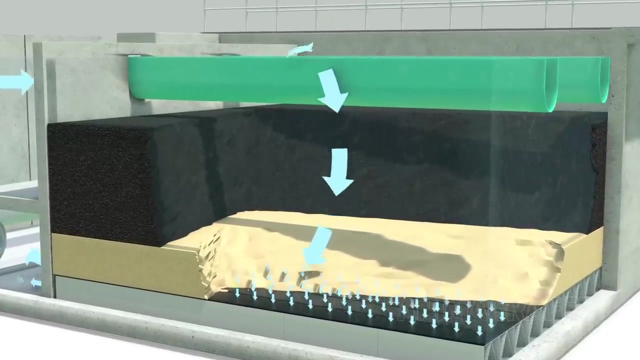 It's called activated carbon because the resulting engineered granules, which are processed from common materials like wood, coal or even coconut husks, have a relatively large surface area with many features and pores, giving ample opportunity for contaminants to catch or stick to the surface as water passes through. 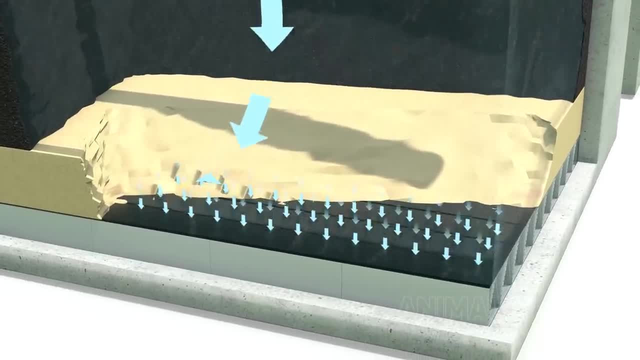 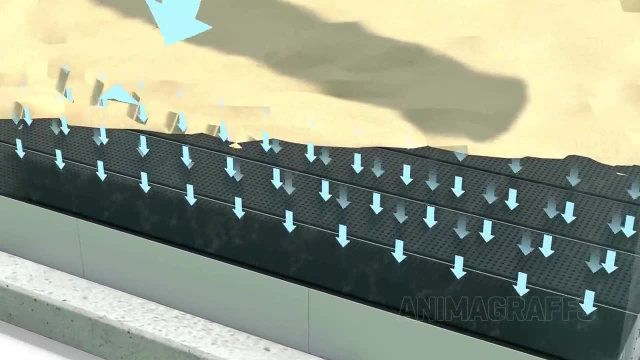 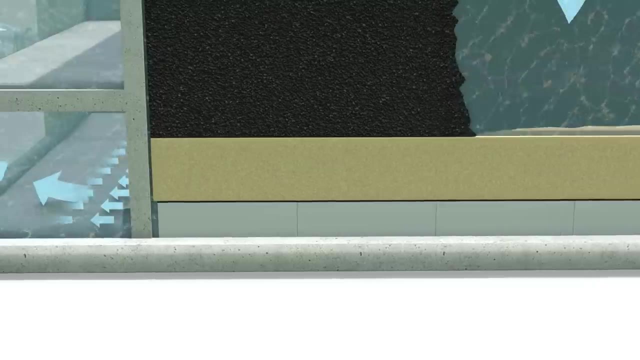 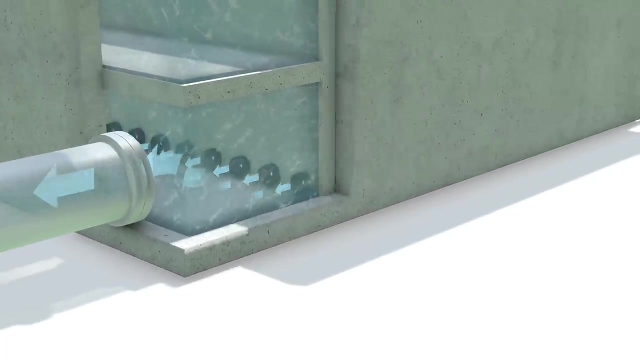 Generally speaking, the activated carbon layer filters biological and chemical elements, while the sand layer filters inorganic elements like unwanted metals. Passing particles stick to a carbon or sand granule surface due to naturally occurring attractive forces called van der Waals forces. The filtered water flows to final disinfection in the UV tank. 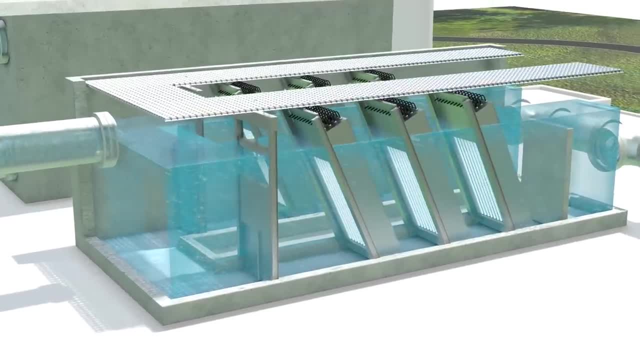 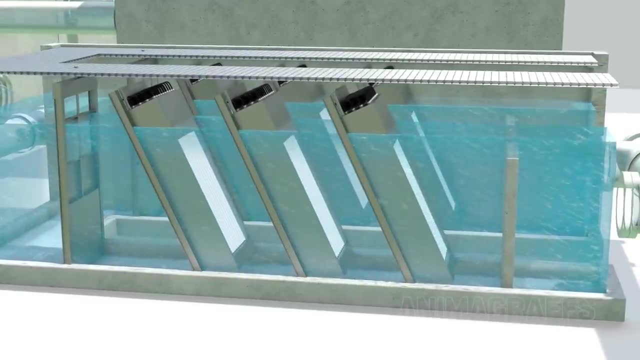 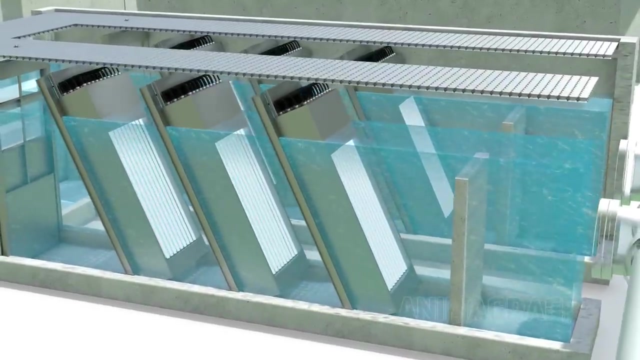 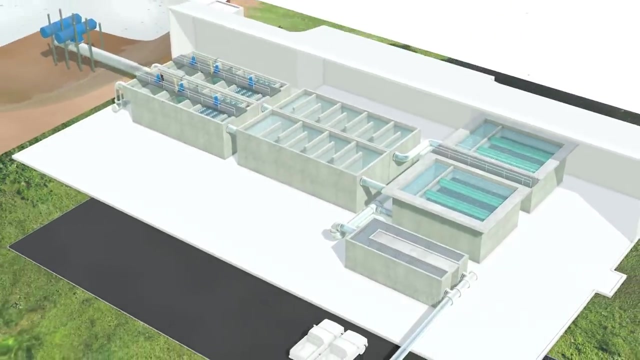 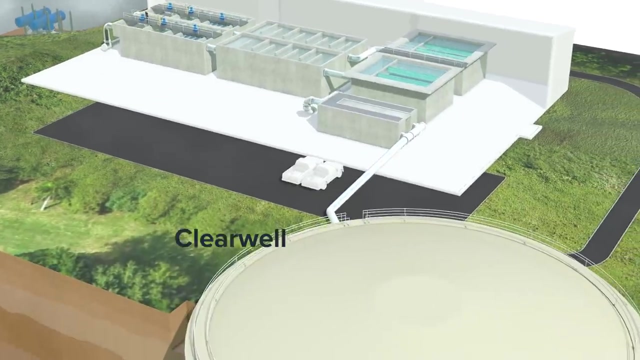 Water passes through banks of ultraviolet lights. UV light at various wavelengths can destroy or disrupt viral, bacterial and other pathogens' DNA or cellular structure, effectively destroying them. The water is now ready for public consumption. It flows into what's called a clearwell for storage. 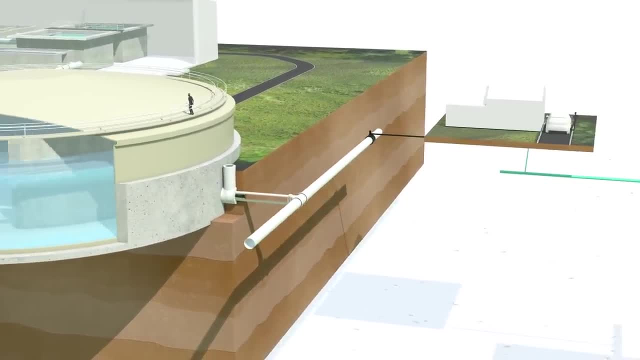 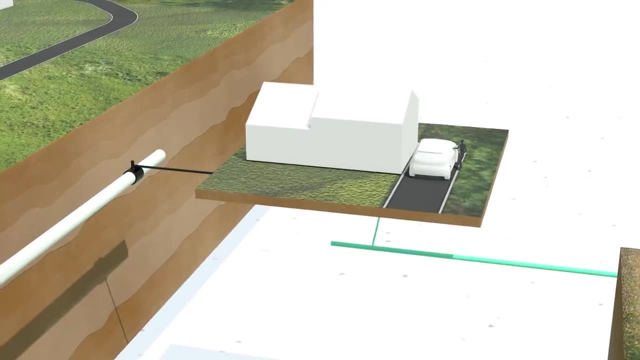 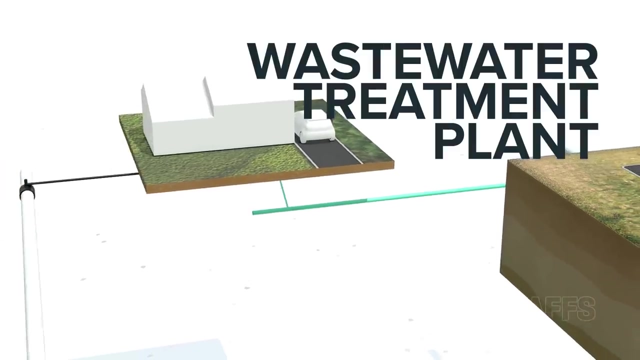 or into the municipal system for use. It can be used to store and store waste water. Now let's look at what happens to water after we use it. What is a clearwell Waste water flows from our homes through the municipal collection system or 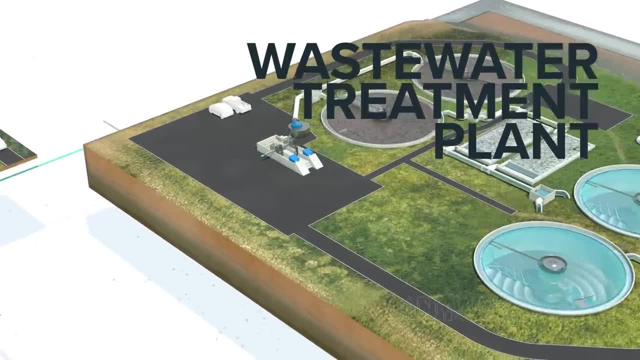 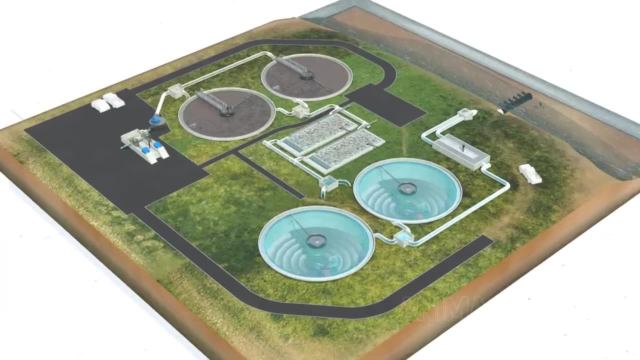 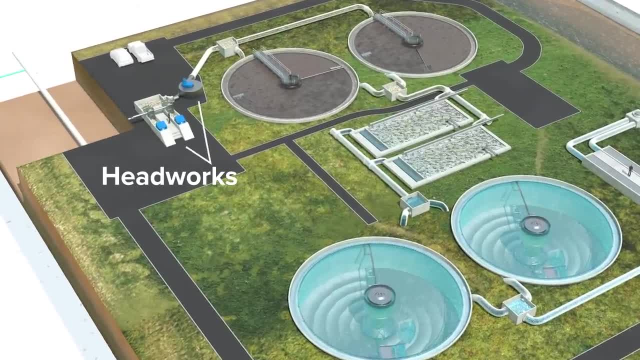 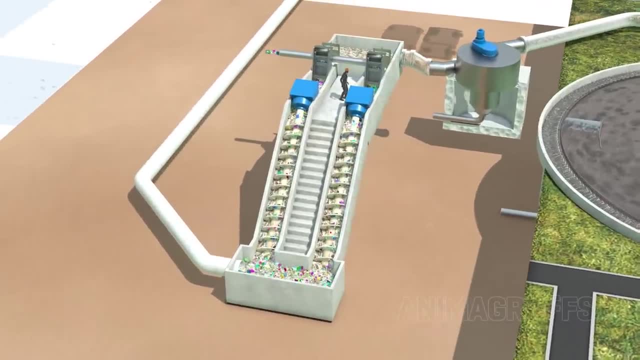 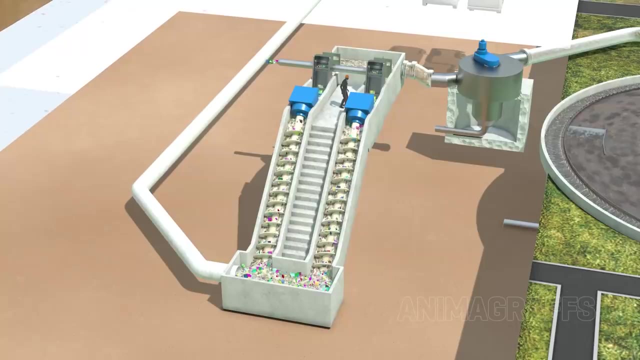 What is a clearwell? What is a clearwell? The headworks is a group of processes that removes large debris and heavier inorganic particles from the incoming wastewater flow. Water arrives at the plant mostly by gravity. Depending on local geography, it may need to be pumped or lifted into the wastewater. 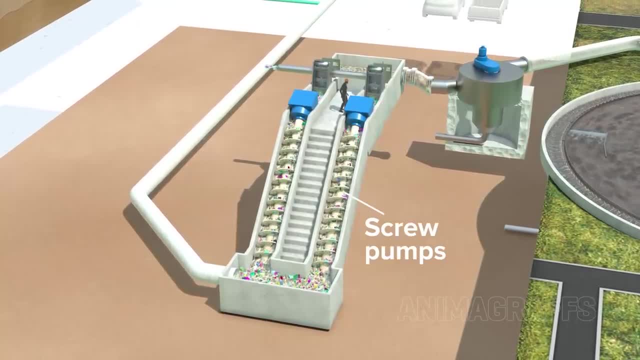 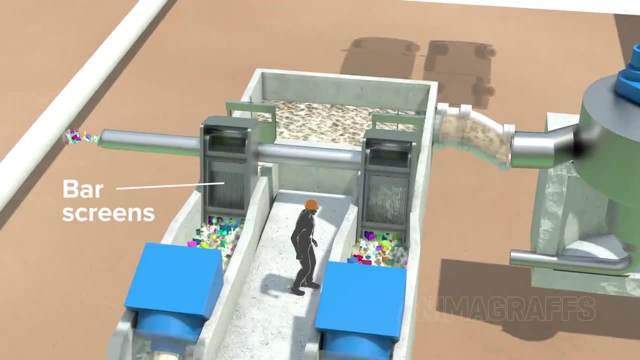 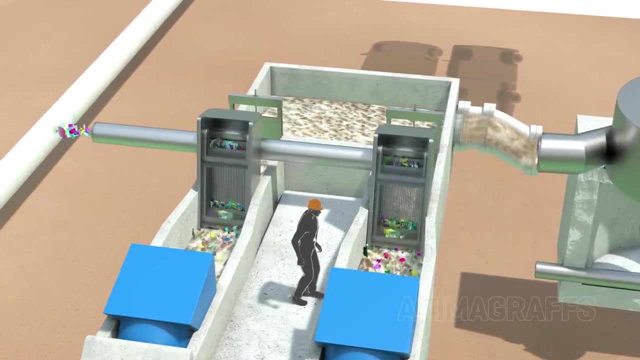 plant Screw pumps are a rugged, mechanically simple design built to handle this coarse incoming mixture. Bar screens, trap debris, including literal tons of items that really shouldn't be flushed or sent down the drain, such as baby wipes, q-tips, diapers, paper towels, medication. 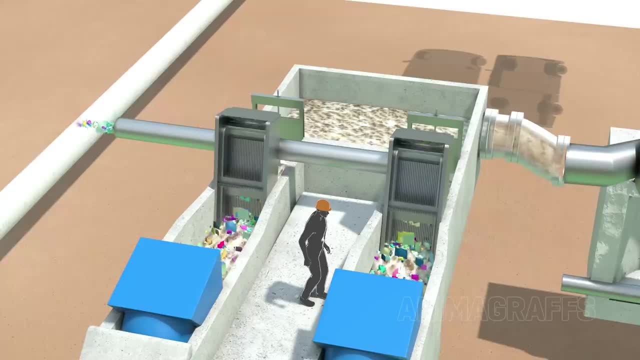 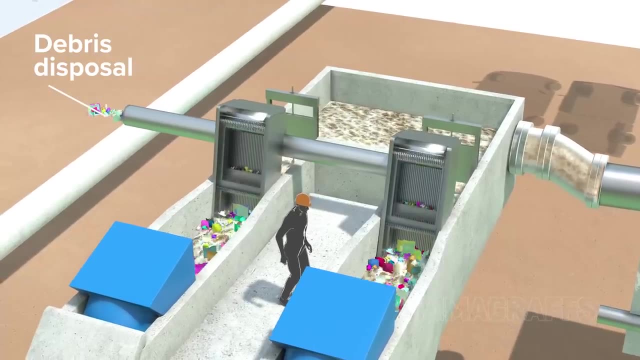 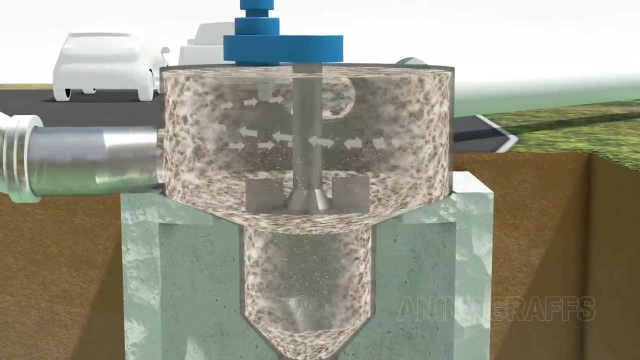 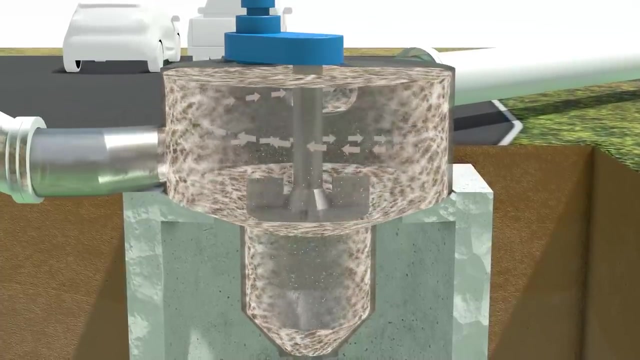 and so on. A moving platform called a rake scrapes the bars, removing the debris for separate processing and disposal. The water then travels to the grit chamber to remove heavier inorganic gritty particles like sand, silt, clay, coffee grounds, eggshells and so forth, while allowing lighter organic. 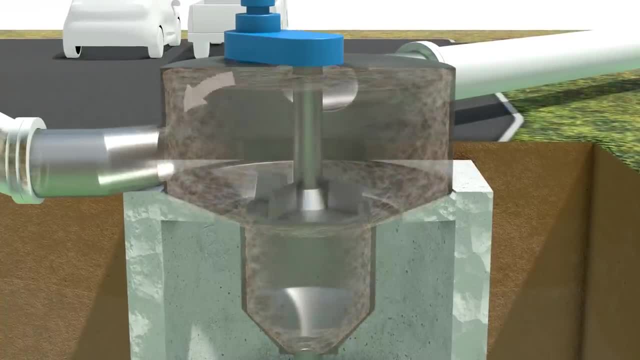 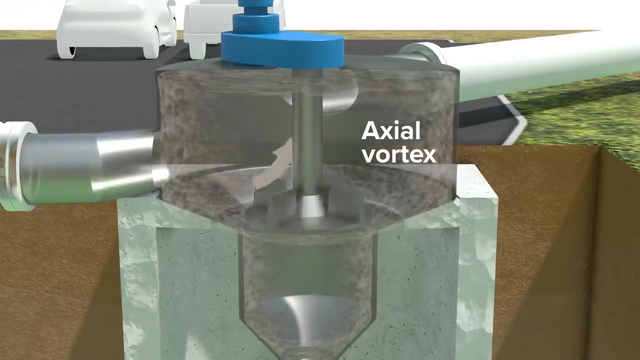 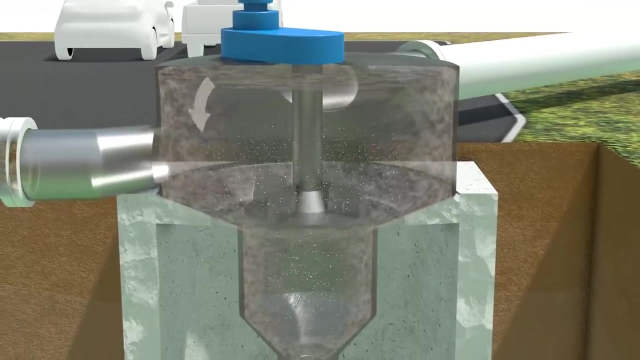 material to pass through A spinning plate with fins called an impeller creates an axial vortex, which is a sort of vertical spiral force along its spin axis at a specific speed so as to catch particles in a defined weight range. These heavier grit particles are forced down the grits and are then transferred to the 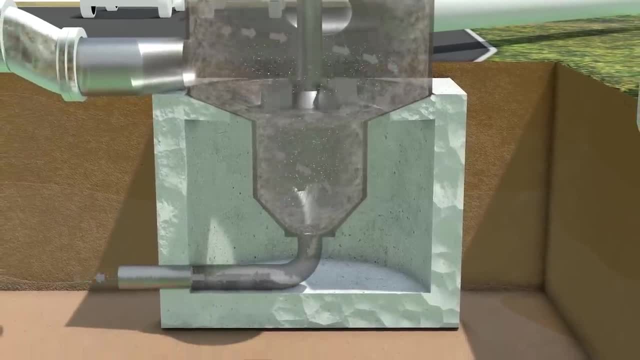 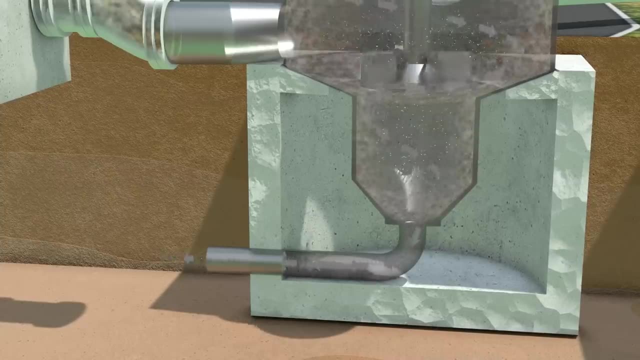 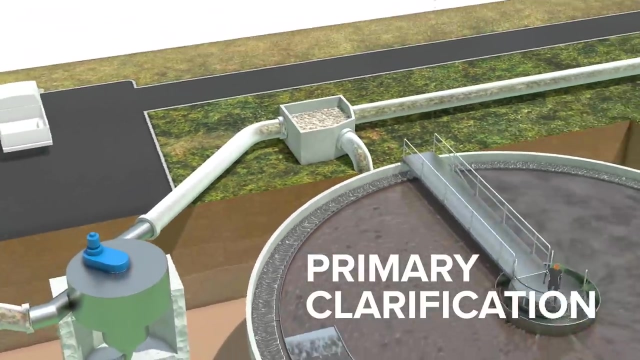 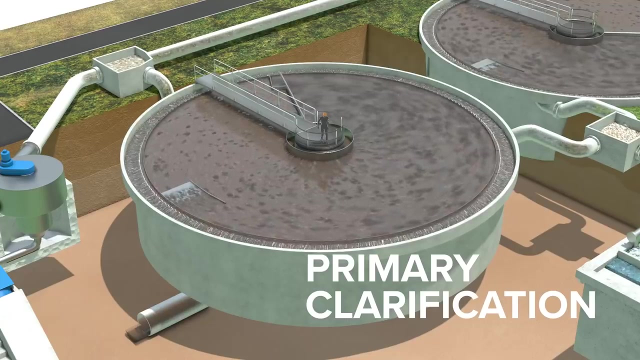 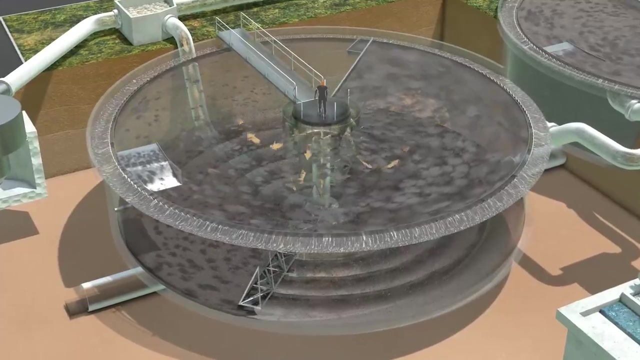 forced-down chamber walls and out at the bottom The grit is collected to undergo its own separate dewatering and washing process. The wastewater leaves the headworks towards primary clarification. Primary clarification separates organic matter from the wastewater. The water flows in at the center of large circular basins called sedimentation tanks. 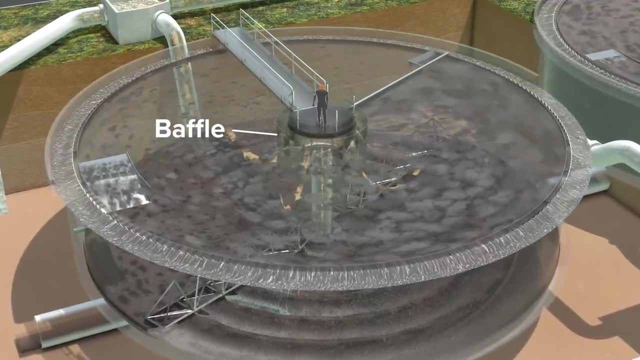 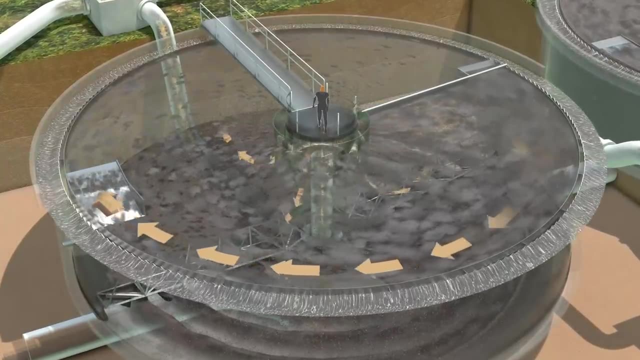 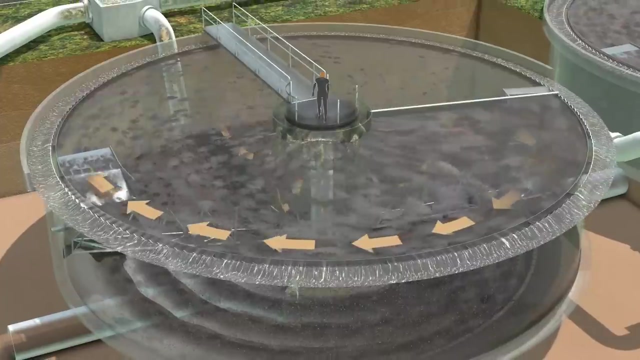 The baffle slows down the flow rate to aid the settling process. Floatable solids like grease and oil drift to the top of the tank. A rotating skimmer continually pushes this material into a collection trough. Settlable solids sink to the angled bottom of the tank and form a sludge. The water flows in at the center of large circular basins called sedimentation tanks. The water flows in at the center of large circular basins called sedimentation tanks. The water flows in at the center of large circular basins called sedimentation tanks. 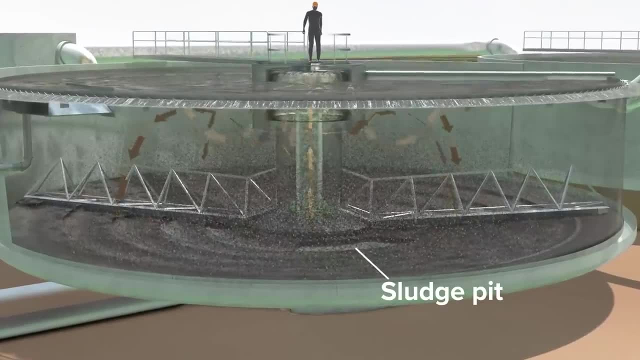 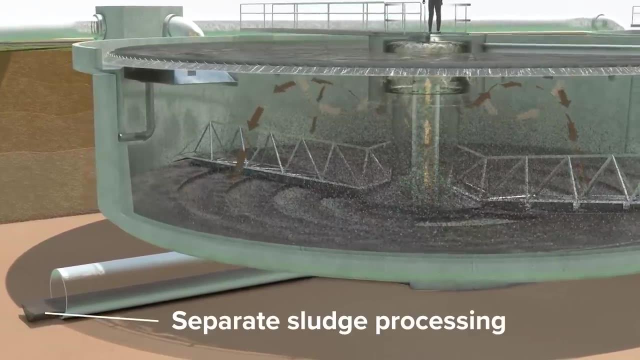 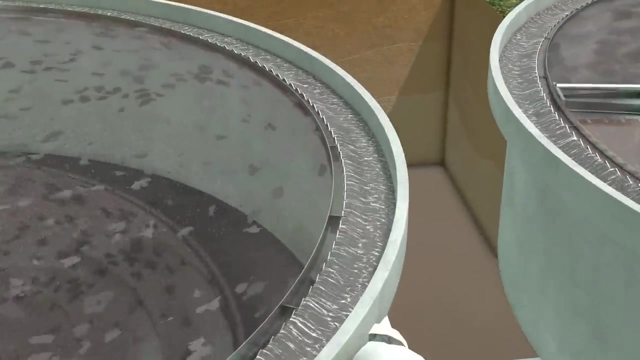 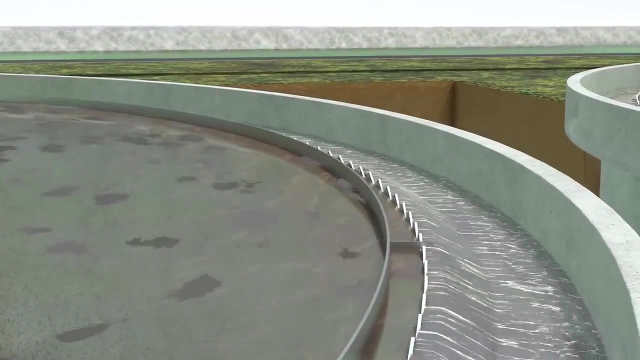 Scraper arms push the sludge out of the tank into a sludge pit. This organic matter has its own purification process and can eventually be used, for example, as fertilizer. A baffle at the edge keeps floating material from mixing with outgoing processed water. 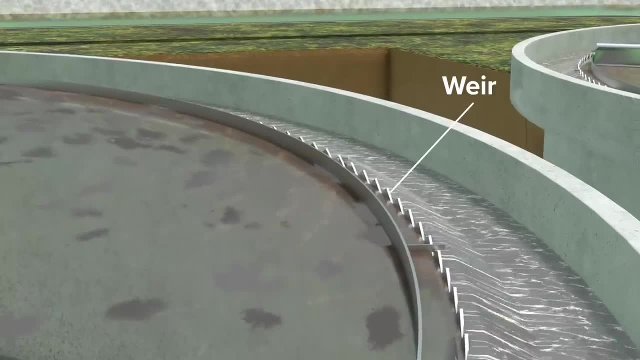 as it flows over a lip at the edge of the tank. The water flows in at the center of large circular basins called sedimentation tanks. The water flows in at the center of large circular basins called sedimentation tanks. This organic matter has its own purification process and can eventually be used, for example. 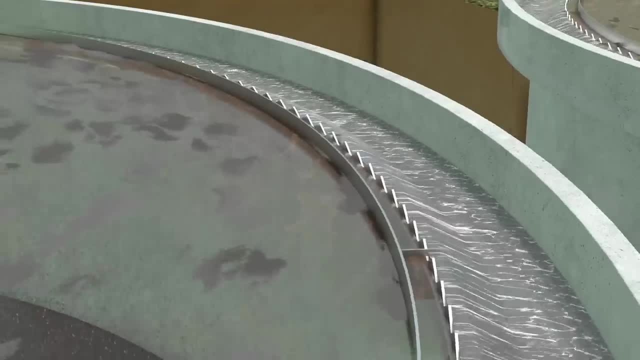 as fertilizer. The water flows in at the center of large circular basins called sedimentation tanks. This organic matter has its own purification process and can eventually be used, for example, as fertilizer. The water flows in at the center of large circular basins called sedimentation tanks. 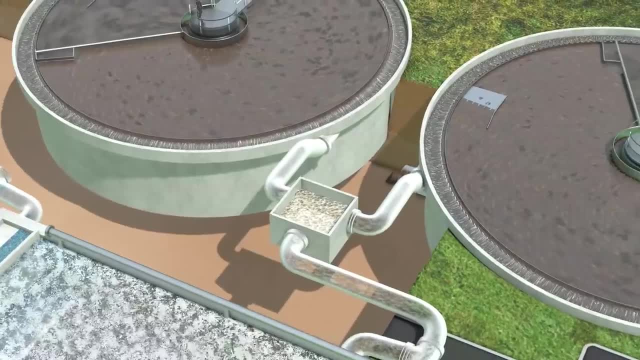 This organic matter has its own purification process and can eventually be used, for example, as fertilizer. The water flows in at the center of large circular basins called sedimentation tanks. This organic matter has its own purification process and can eventually be used, for example. 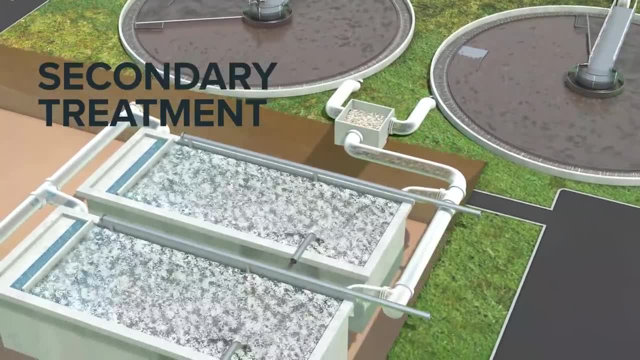 as fertilizer. The water flows in at the center of large circular basins called sedimentation tanks. This organic matter has its own purification process and can eventually be used, for example, as fertilizer. This organic matter has its own purification process and can eventually be used, for example. 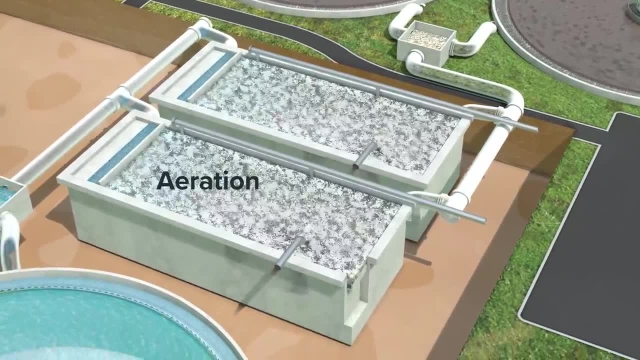 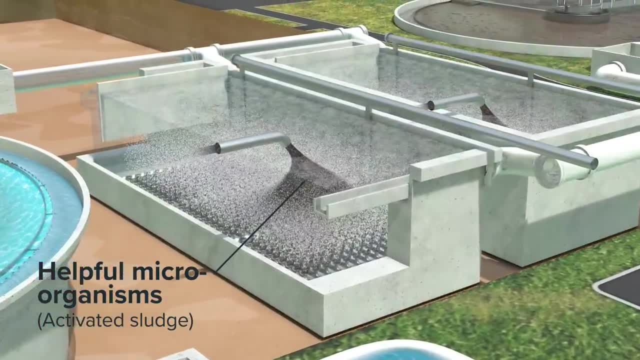 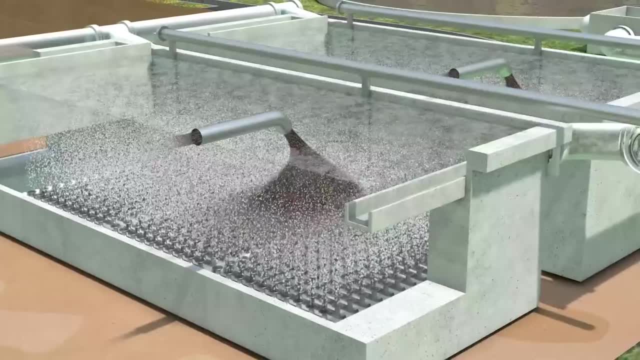